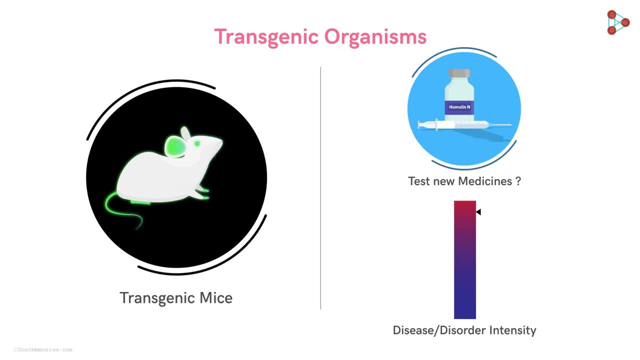 organisms, then testing medicines will not be possible. So how will new medicines be discovered and used? That indicates the need of using model organisms. So what should be done? ideally? There is no single answer for this, actually, And hence for these types of concerns, we have the fields of: 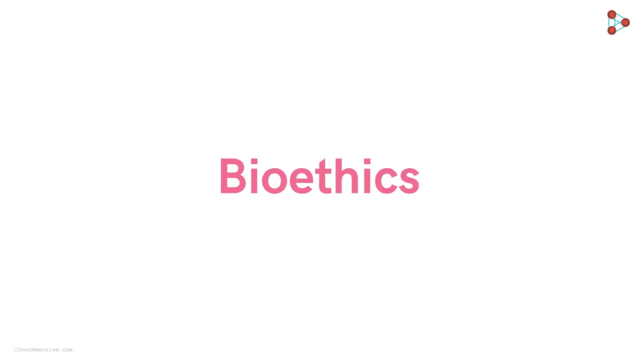 bioethics. Now let's first understand what bioethics is. It's simply the area dealing with ethical issues in the field of bioethics. So what is bioethics? Well, it's a field of bioethics that is used in the field of medicine or any other biological studies. In this video, let's learn. 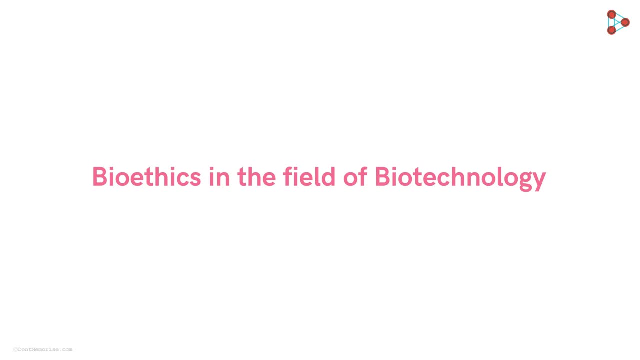 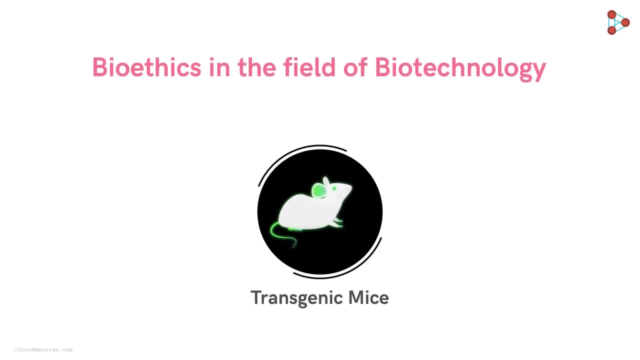 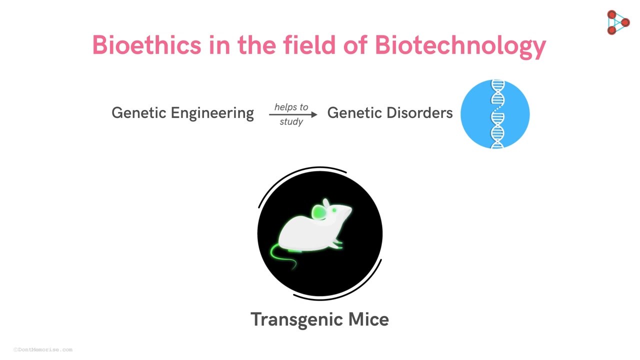 about bioethics in the field of biotechnology. Let's begin with the same point that we discussed a few minutes ago: Transgenic organisms. Genetic engineering enables us to study the various genetic disorders And, for these types of studies, transgenic animal models like the transgenic mice. 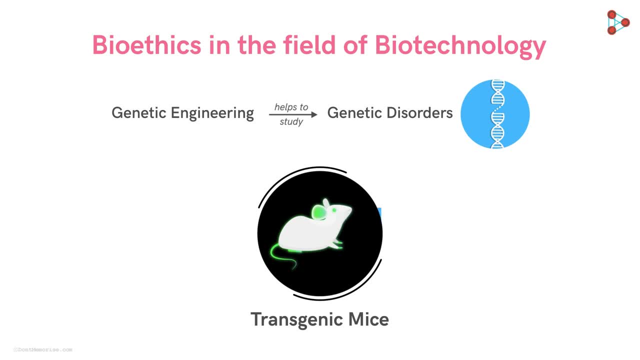 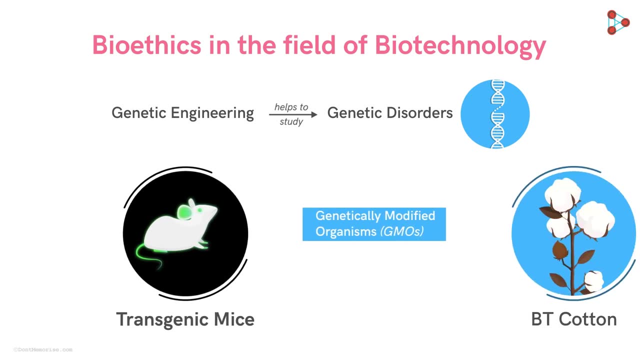 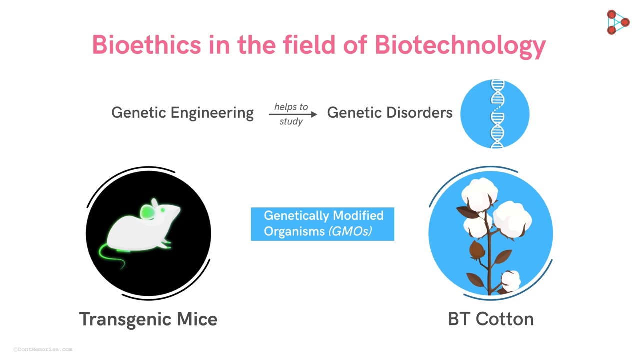 are developed. These animals, as we know, are called genetically modified organisms or GMOs, And just like animals, plants are also modified. So the transgenic crops produced, too, have qualities that we desired. Just like the golden rice, for example, it contains wholesome amount of beta carotene. 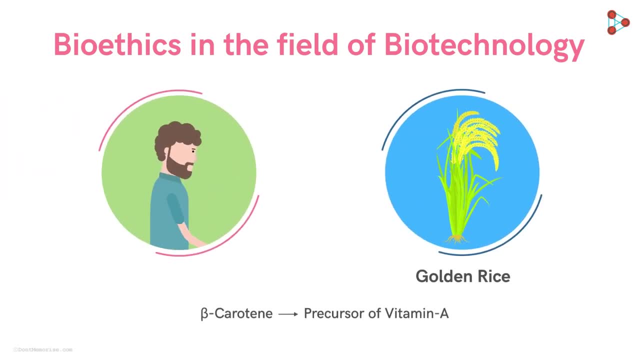 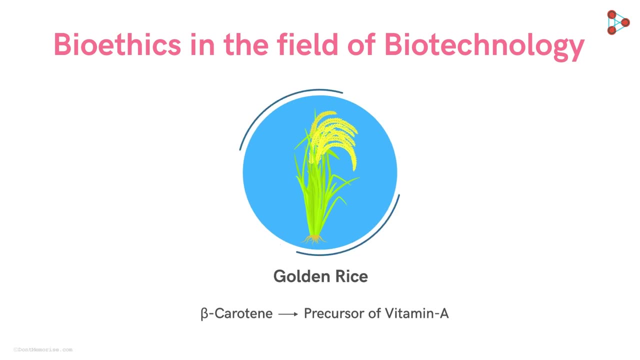 which is the precursor of vitamin A. When consumed, the compounds get converted to vitamin A in the body. The transgenic rice variety is a boon to areas hit with vitamin A deficiency, But if the organisms are so beneficial to us, then is their production really an ethical concern? 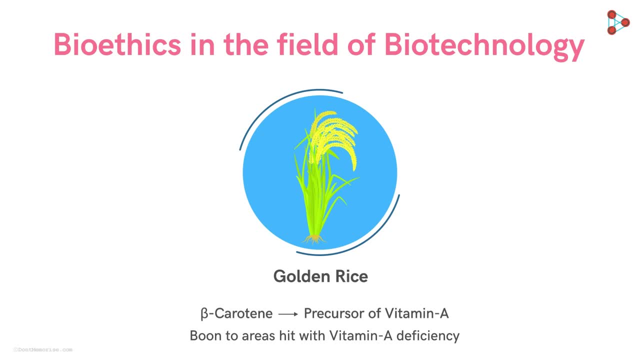 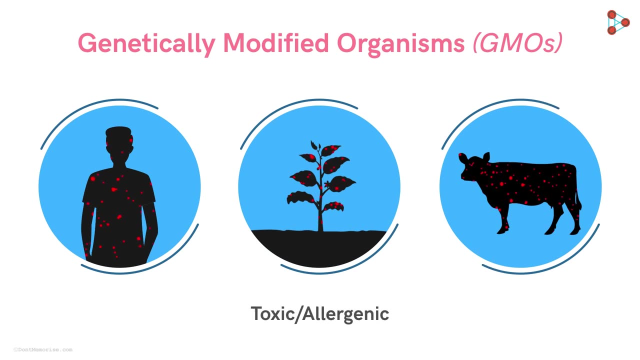 Yes, that's the other side of the coin. GMOs are known to produce several compounds, among which a few can be toxic or allergenic in nature. We cannot ensure that these untraced compounds would not harm us. Thus, there are several hidden risks attached to it. 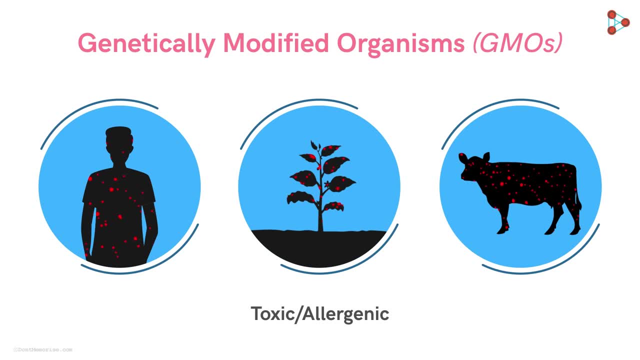 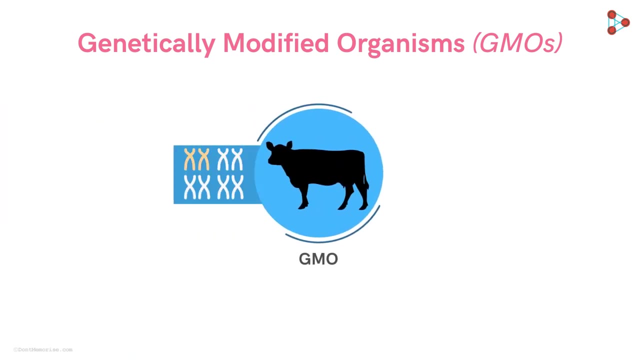 There can be possibilities that the GMOs turn out to be actually more harmful rather than being beneficial. The long-term side effects of GMOs are still unknown, Also as we know that transgenic organisms have a completely different gene pool from the wild varieties. 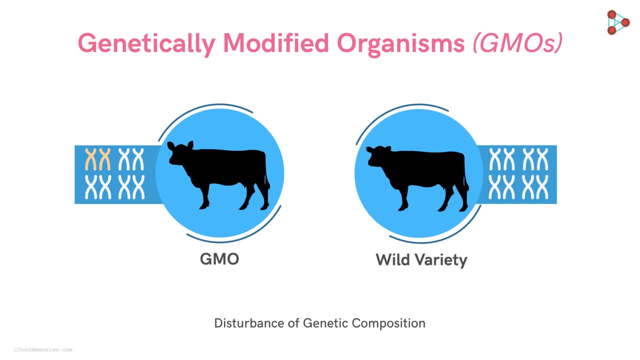 So at the species level, we disturb the genetic composition of those organisms. Do we really know what impact this can create several years later? What can happen if the transgenic genes sustain in the gene pool forever? And what if the natural genes are lost? 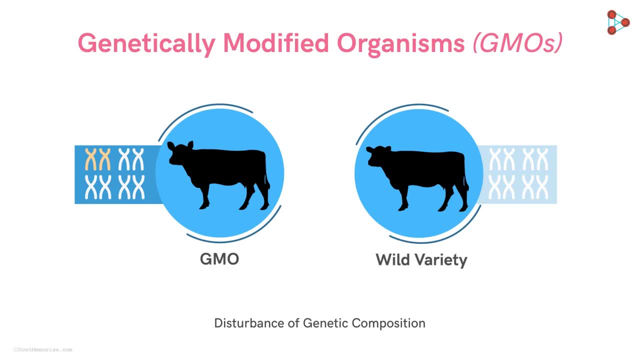 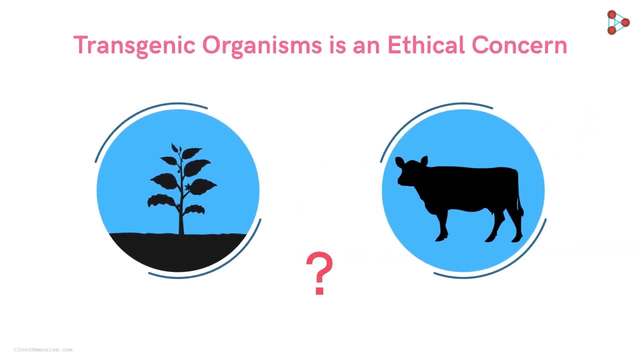 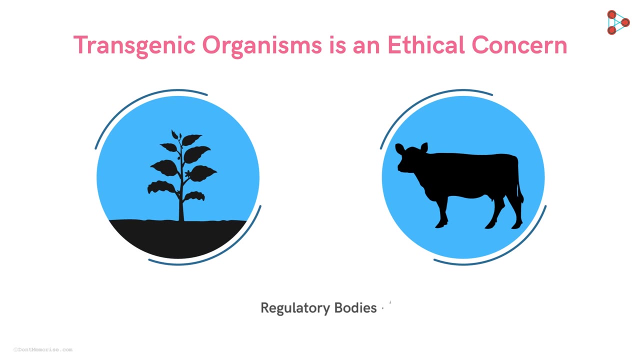 There are many other questions that emerge as we go deeper into this discussion. Hence, making transgenic organisms is an ethical concern. So what's the solution to this? There is no fixed solution for this, But, yes, there are few. There are a few regulatory bodies which glance at the various activities in the field of biotechnology. 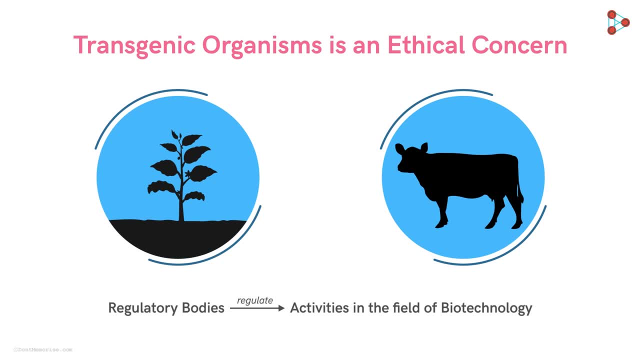 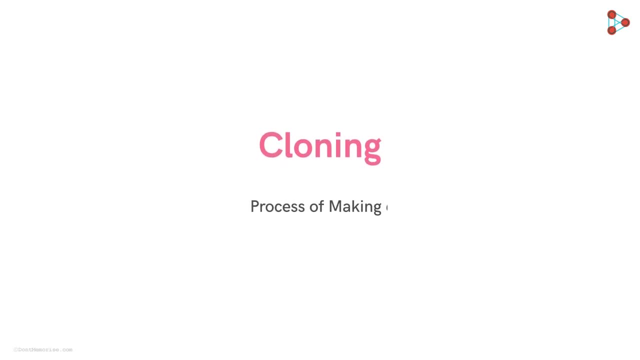 Now let's talk about one more hot topic in bioethics, and that is cloning. We know that cloning in biotechnology deals with the process of making exact copies of biomolecules or organisms. How about human cloning? The idea sounds cool, but that is not so great in reality. 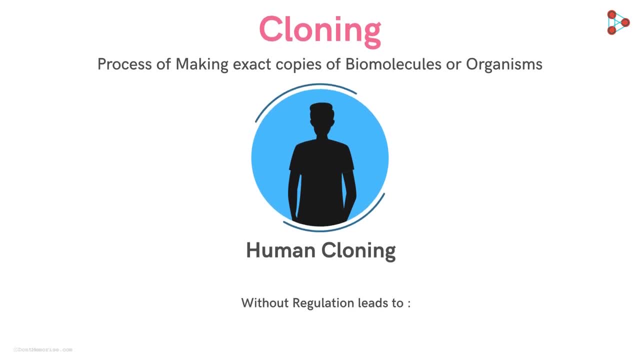 Preparing human clones without regulation would definitely lead to serious concerns like overpopulation, increase in diseases, exhaustion of limited resources and many more. Also, this can act against the balance of nature. We know that nature promotes variation in the gene pool of organisms. 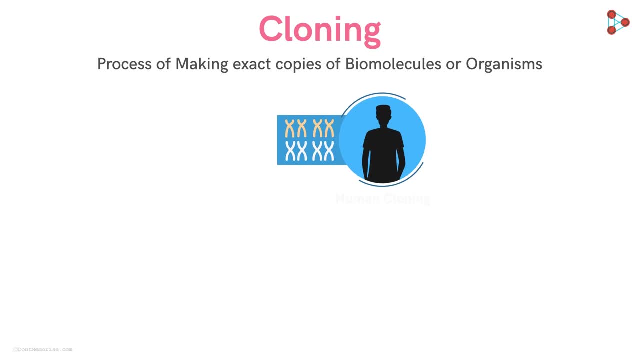 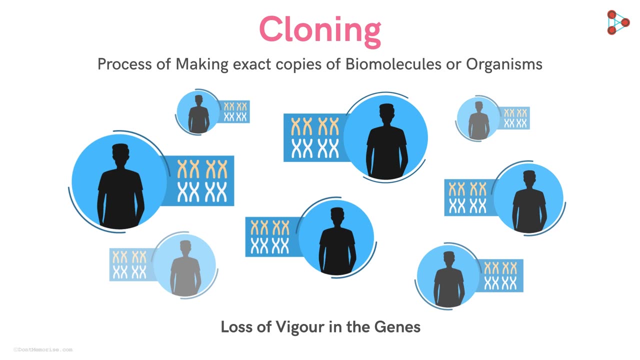 Cloning can lead to utilization of the same gene pool constantly, thus leading to a loss of vigor in the genes, And there are many other issues which pop up with the process of making clones. Thus, the question whether cloning is favorable or not still remains unanswered. 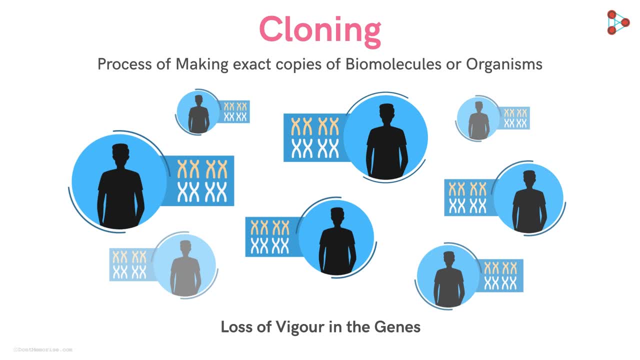 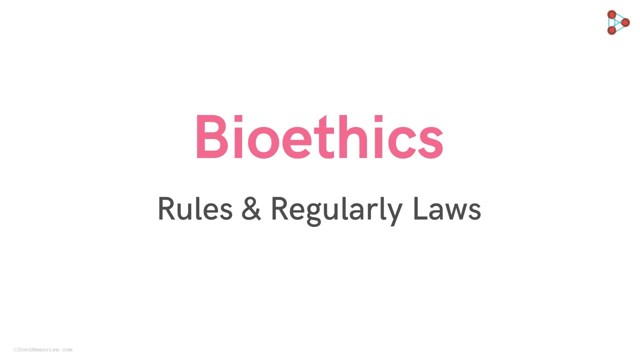 For all such questions, which literally churn our minds, the only option that comes to our rescue is bioethics. There are several rules and regulatory laws laid under bioethics that help us make wise decisions as we stumble upon heart-wrenching obstacles. For more information on bioethics, please visit our website at wwwbioethicscom.